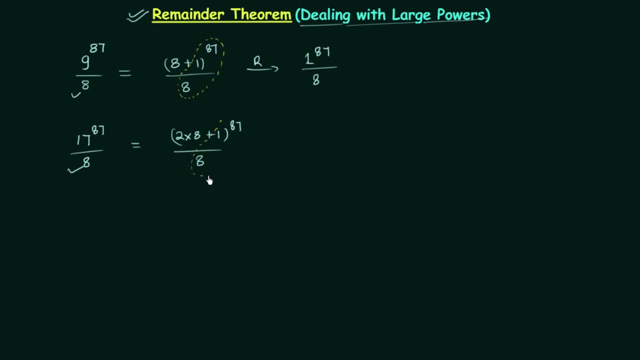 8.. And in this case also we will do the same thing: 1 raise to power- 87 over 8.. You don't have to worry about this first term. So we already know: 1 raise to power- anything is going to be 1.. So 1 raise to power- 87 will be 1.. So we have 1 divided by 8 and the remainder 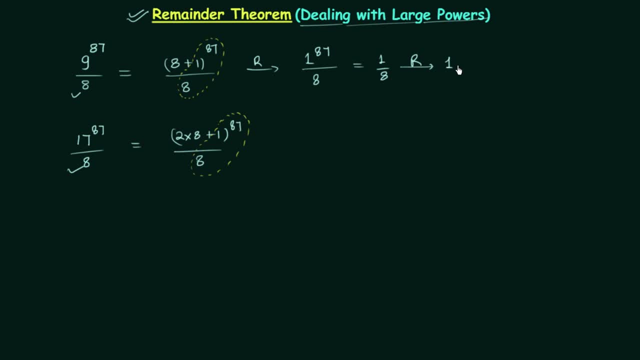 of 1 divided by 8 is 1.. So we can directly write down answer as 1. if we can directly proceed to calculating the remainder of 1, raise to power 87 over 8. And break the numerator like this. In this case also we can directly write down the answer. 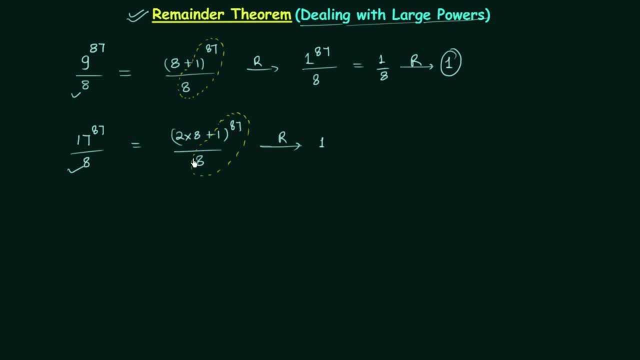 as 1.. Now we will see the proof of this method, but first I will generalize. I will generalize this method: If you can express the expression in the form, in the form bx plus 1, raise to power n over x, then you can directly write down the remainder as 1.. 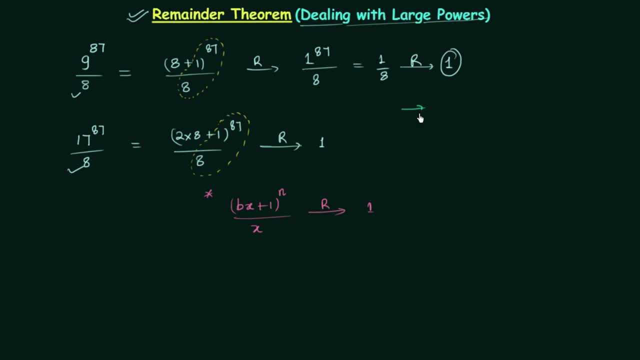 You have to remember this. Now we will see the proof of this method. Let's say we have x plus a raise to power n and we can write this as x- raise to power n plus nc1 x- raise to power n minus 1 a raise to power 1.. The next term is nc2- x- raise to power n- minus. 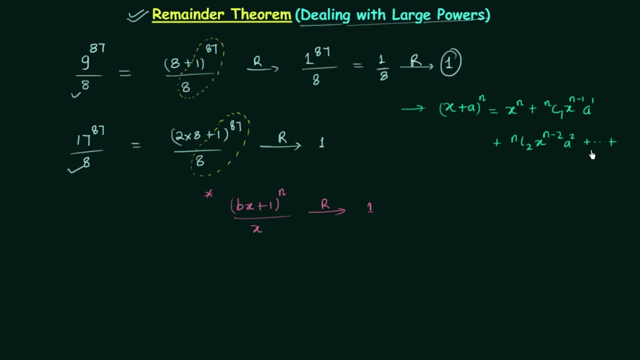 2: a raise to power 2.. Plus all the way to ncn x: raise to power n minus n and a raise to power n, And you can write the last term as a raise to power n. So I will write it as a raise to power n only. 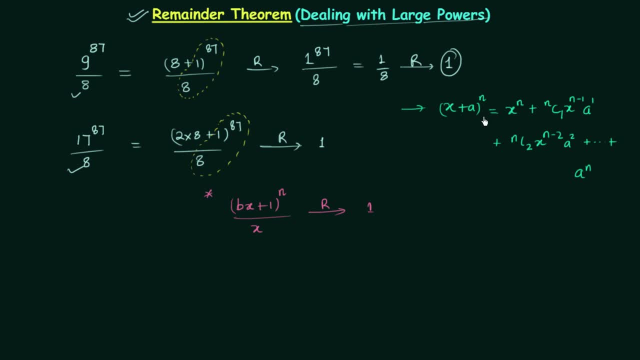 So this is the expansion, And now I will divide x plus a raise to power n by x. I will divide it by x, So the right hand side also. I will divide it by x, So the right hand side also. I will divide it by x. Now, if the first term, which is x- raise to power n- is divided by 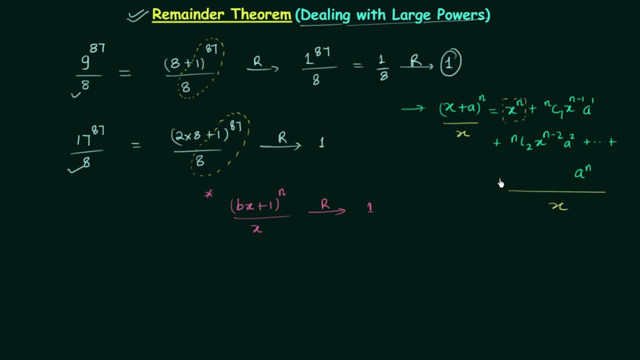 x, you are going to get the remainder as 0 because we are having x in the numerator. In the same way, here we are having x raise to power n minus 1.. When you divide it by x, you will definitely get remainder equal to 0.. In the same way, you will get remainder. 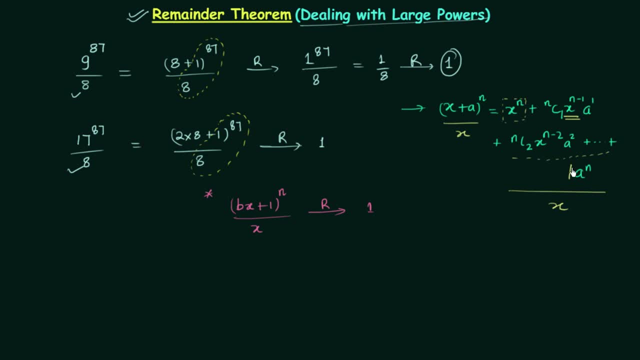 equal to 0 for all the terms except a raise to power n. So the final remainder is a raise to power n minus 1.. So the remainder is a raise to power n minus 1.. So the remainder you are going to get will depend on the last term. 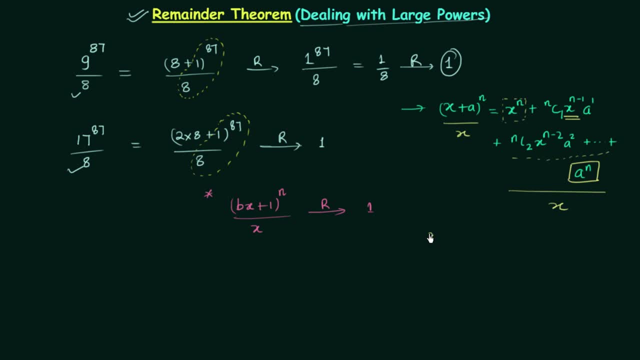 only So what I can write. I can write: when x plus a raise to power n is divided by x, the remainder is going to be the remainder of a raise to power n by x. I will write remainder of a raise to power n over x. So in this way you can easily prove this method. 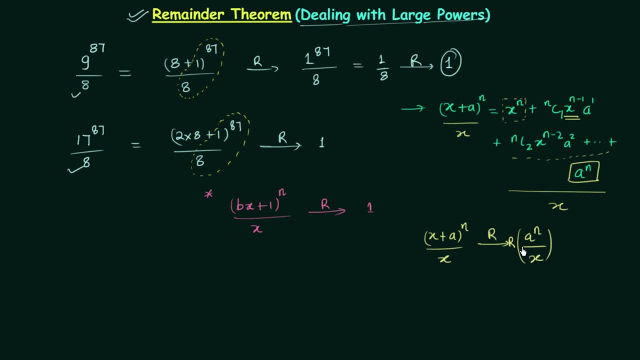 I will check the first example by using this. Here you can see you have 8 plus 1 raised to power 87 by 8.. I will write 8 plus 1 raised to power 87 by 8, so 8 is x. You can see 8. 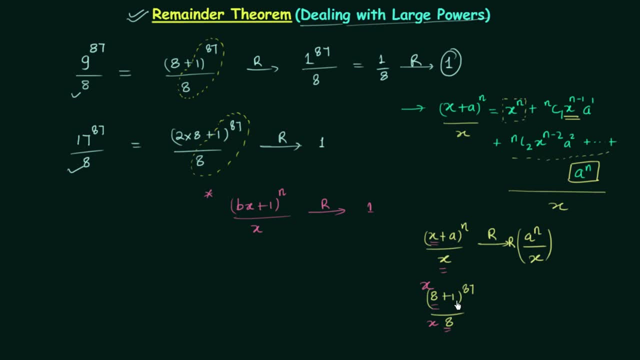 is x and a is 1.. n is 87. So the remainder is going to be. So now you can use the second method. let me use the second method. So 8 plus 1 by 8, you have 8 plus 1 raise to power. 87 by x by Bott, So 8 is x. you can see 8 is x and is 1 by 87. So the remainder is going to be 8 plus 1. raise to power n is 87. So that is eight. Now it will be zero Now the 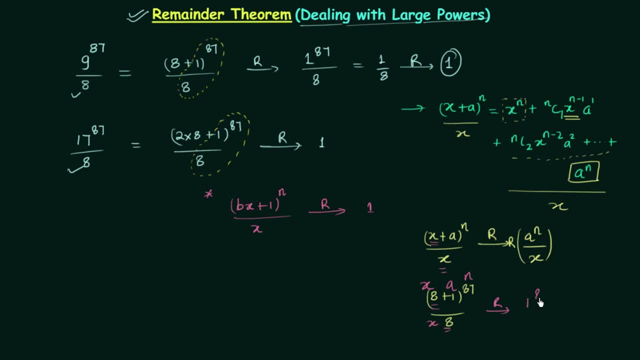 a raise to power. n. a is 1, so 1 raise to power 87, because n is 87. divided by x, x is 8 and the remainder you are going to get is 1, because 1 raise to power anything is equal to 1 and 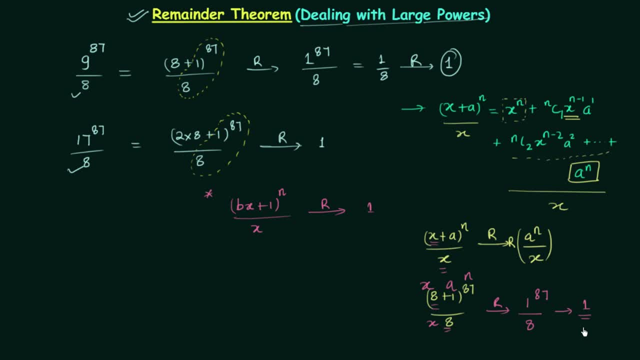 1 divided by anything will produce the remainder equal to 1.. So this is how you can have the complete explanation of this process. Now we will quickly solve few more examples related to this method. In the first example, 37 raise to power. 1,, 9,, 3,, 7, 6 is divided by 9.. Now 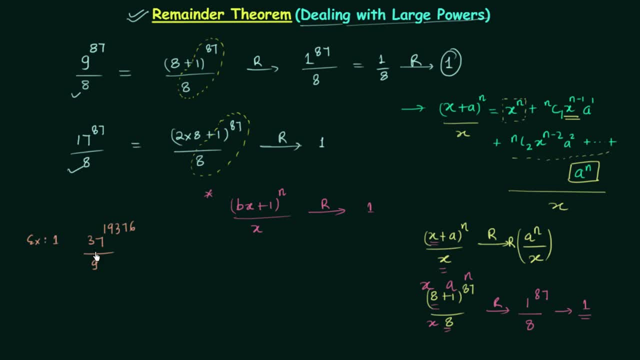 you have to think how you can break 37 so that you have the form bx plus 1.. Right, So let's try to think about it. 9 multiplied by 4 is equal to 36, and 36 plus 1 is 37. Pretty. 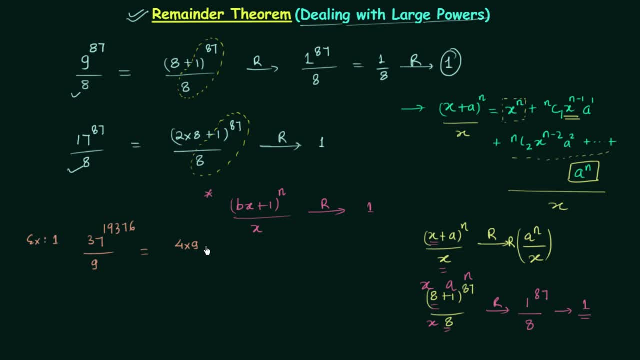 simple. So 4 multiplied by 9 plus 1, the power is 19376, 19376 divided by 9.. So we have this form and we can directly write down the remainder as 1.. So remainder is going to be 1.. This 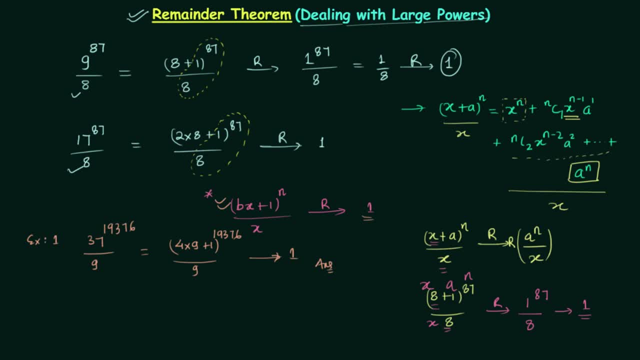 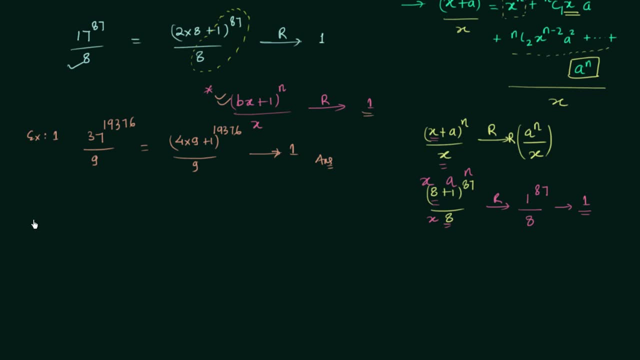 is the answer. Now what if you cannot directly obtain this form? The problem will be very difficult in that case, But if you think In correct direction, you can easily solve that kind of problem also. Let's take another example in which we will deal with such case. 9 raise to power 100 is divided by 7.. Now 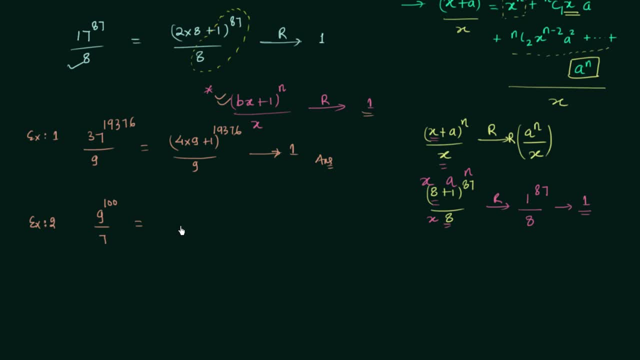 if you try to break 9 in this form, you cannot break it because 8 plus 1 divided by 7 is not this form, because we need 7 in the first term. So let's try to break it like this: 9 raise to power 100 is divided by 7 plus 2 raise to power 100 over 7.. Now, if you follow, 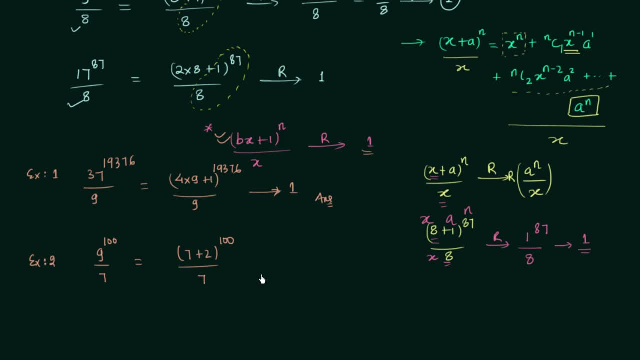 if you follow this expansion, you can clearly get the result in which the remainder will only be dependent on last term, which is 2 raise to power 100.. So the remainder will depend on 2 raise to power 100 divided by 7.. And I can write 2 raise to power 100 as 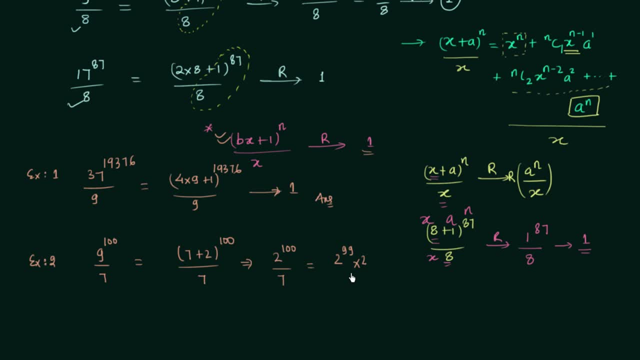 2 raise to power 99.. 2 raise to power 99 multiplied by 2, divided by 7.. 2 raise to power 99, I can write as: 2 raise to power 3. raise to power 33, multiplied by 2, divided by 7.. 2 raise to power 3 is equal. 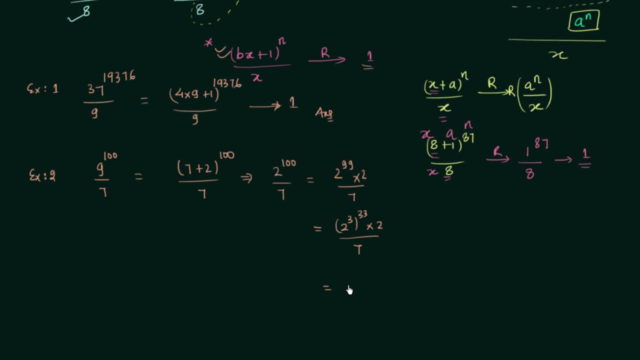 to 8.. 2 raise to power 3 is equal to 8.. So 8 raise to power 33, multiplied by 2, divided by 7.. Now I can write 8 as 7 plus 1.. is this form? so we have 7 plus 1 raised to power 33, multiplied by 2, divided by 7, now we have two.